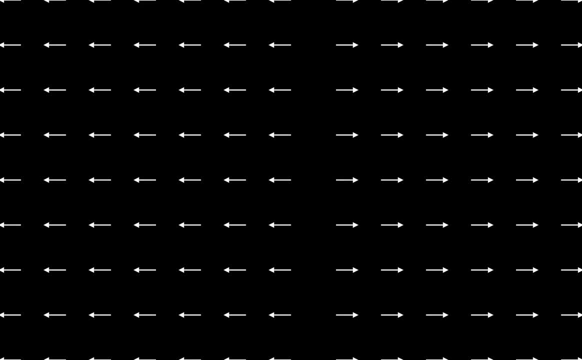 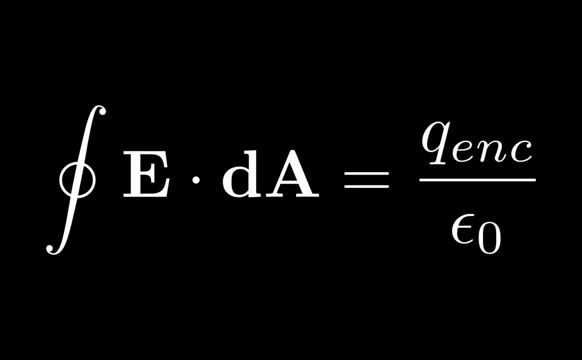 can analytically determine how the electric field will be generated. To do this, we need a method to determine the net charge in an area. Rather than beginning with the differential form of Gauss's law, we'll discuss the integral form first, which looks more complicated but is 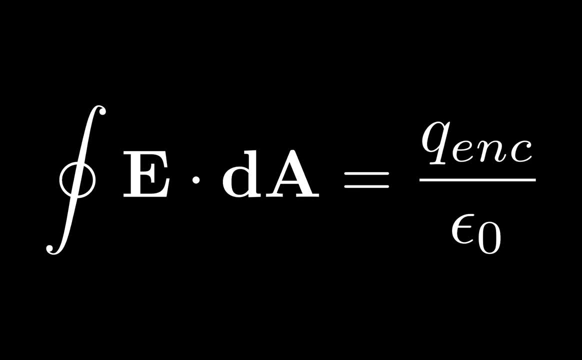 actually more intuitive and arguably more useful For calculus novices. taking an integral is basically just summing up something over an interval using very tiny pieces. We need to take a specific type of integral, in this case to use Gauss's law on the integral form. 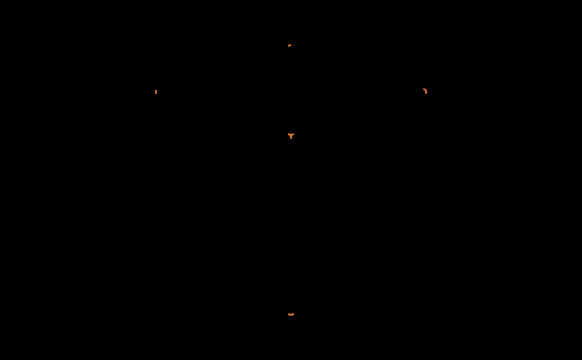 called a surface integral. We'll start by defining a 3D object inside the vector field, for example a cube. However, for the sake of visual clarity, we'll project this surface onto a 2D plane, so it looks like a square on a piece of paper. We can then define vectors, which I'll 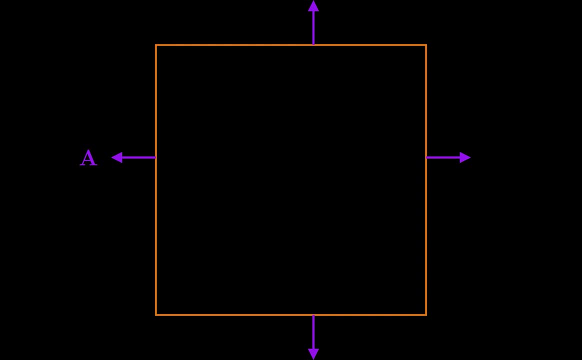 call a that are perpendicular to the surface area of our cube. If we add up the electric field that is perpendicular to every point on the surface, Gauss's law tells us that the sum will equal the charge we've enclosed in that surface, divided by epsilon naught. 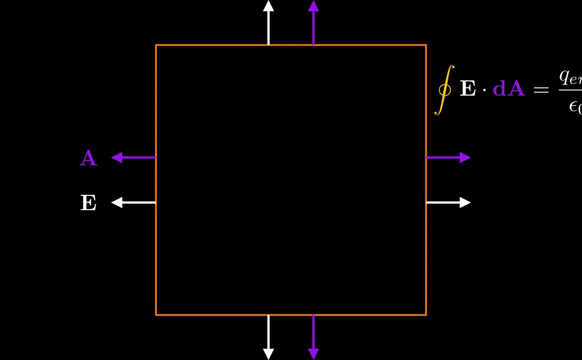 which is a constant that describes how electric fields propagate through a vacuum. You'll often hear that the amount of electric field moving through a surface is referred to as electric flux. If the flux through a surface is positive, Gauss's law says that there must 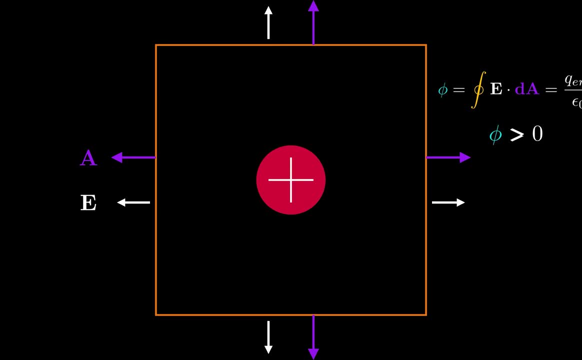 be a net positive charge enclosed. If it is negative, there must be a net negative charge enclosed. We can apply Gauss's law to a variety of electric fields as a kind of charge meter, For example. consider the electric field on screen. now Let's take our charge meter and 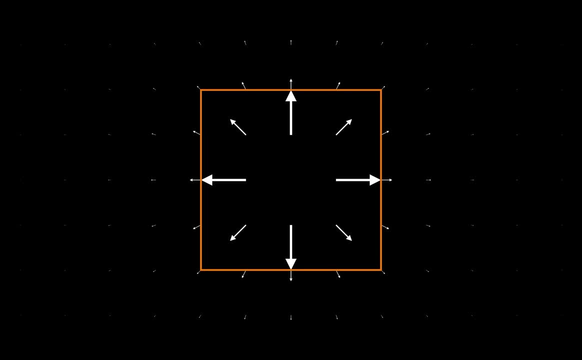 move it to the center of the field, We can visually tell that more field is leaving the volume that we've enclosed than the field that's entering it. Therefore the flux is positive. so Gauss's law tells us that we must have enclosed a net positive charge. 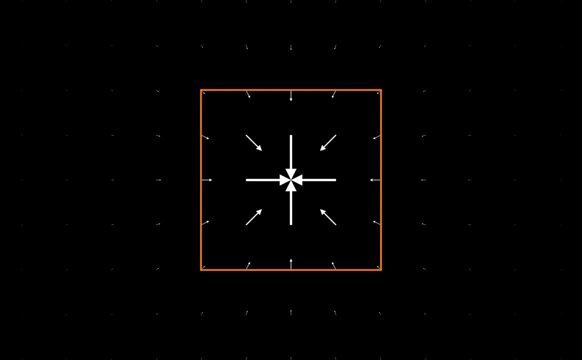 What if we reverse the field? As you can see now, more field is entering than leaving our surface, so the flux is negative. Therefore we must have enclosed a negative charge. Now comes the most counterintuitive piece of Gauss's law. What if we move our solid away? 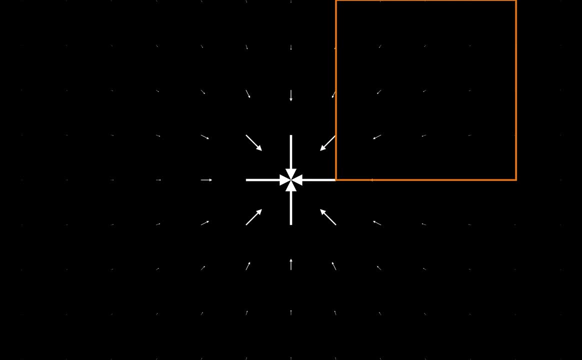 from the center of the field off to the side. Now we can see that we've enclosed a negative charge from the left side of the field off to the center of the screen as well. However, this is not the case. Why? Because the same 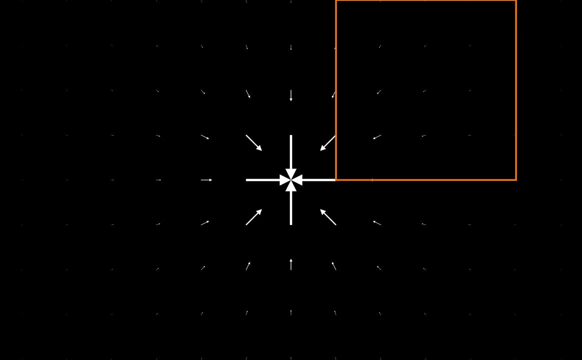 amount of field is moving into the volume, as is leaving it At the flux is zero. Gauss's law says there is no charge enclosed With this newfound understanding, we can now go back to the original field from the beginning of the video. It should be a little clearer now why the original field has no net charged. 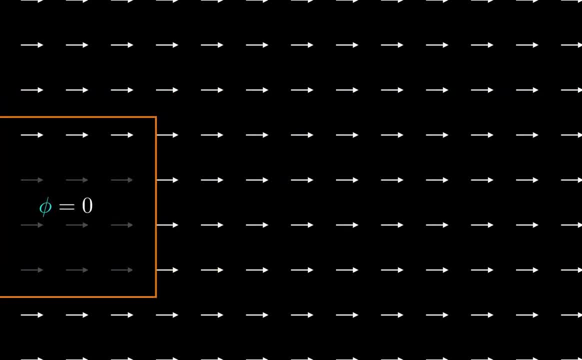 enclosed anywhere on screen, Because anywhere you put our solid, the same amount of field is leaving the surface as is entering it. reversed: half the screen. we create a line down the middle of the screen where more field leaves our solid than enters it, which means that we must have introduced a net positive charge. 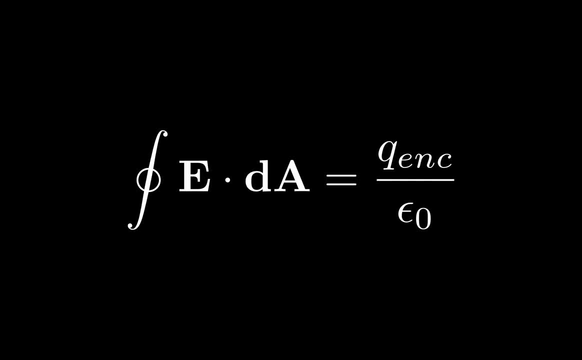 Now that we have a better understanding of the integral form of Gauss's law, we can take a stab at the differential form. This will require some vector calculus ideas. First we need to briefly introduce the gradient or del operator. There are hundreds of hours of fantastic content explaining 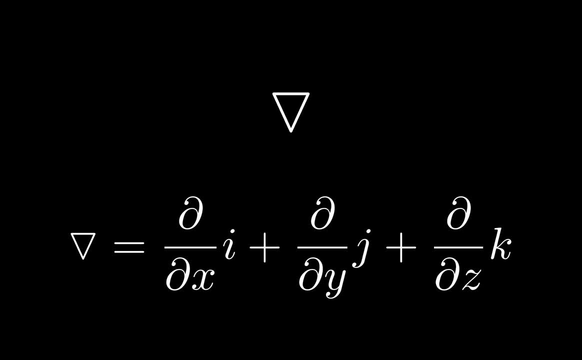 the gradient on the internet, so I'm not going to go into it very deeply. For our purposes, we can think about it as an operator that we can apply to vector fields. When we apply the gradient to a vector field via the dot product, we get the divergence of the vector field, Just so we're on. 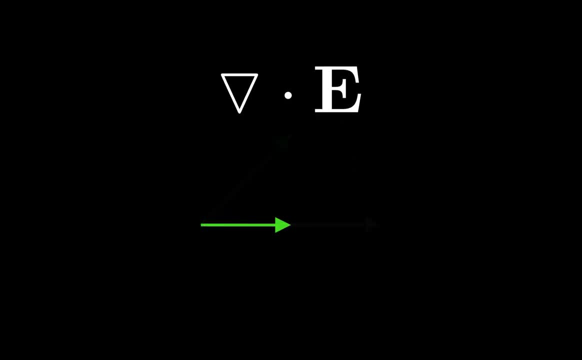 the same page, the dot product tells us the component of a vector that is parallel to another vector. The specific math is fascinating and worth learning, but you don't need to understand any of what just happened to appreciate the meaning of the differential version of Gauss's law. 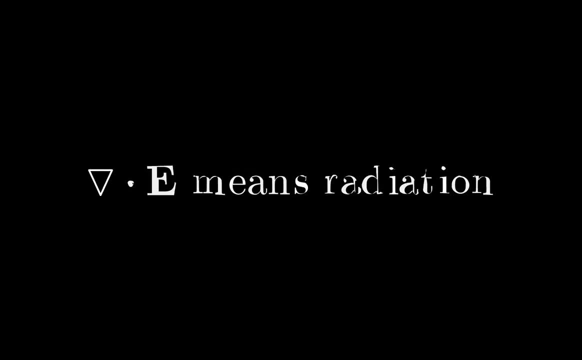 Divergence in this case is a function of the differential version of Gauss's law. In this context, just means radiation. If the divergence is a positive number, it means that the field is radiating outwards. If the divergence is negative, it means that the field is radiating. 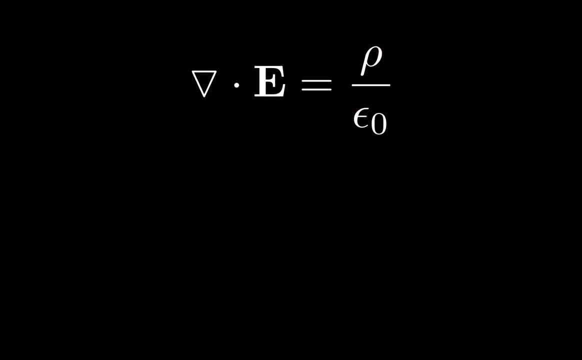 inwards. The differential version of Gauss's law then just tells us that the charge density at a point equals the radiation of the field at that point. If we have a positive charge density, the field will be radiating outwards. If we have a negative charge density, the field will be. 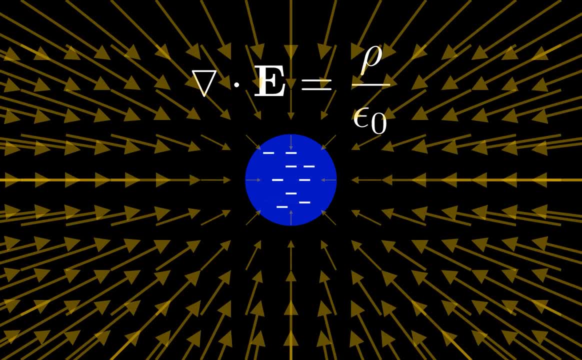 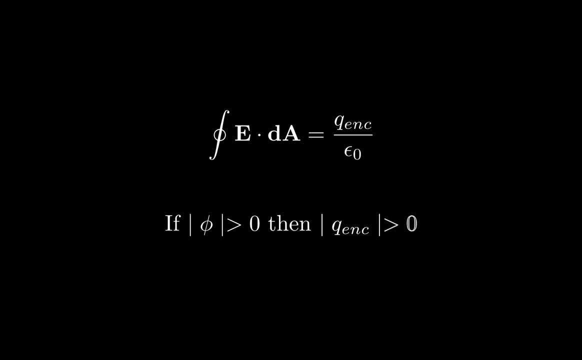 radiating inwards. The larger the density, the more a field radiates. In summary, Gauss's law tells us that if more field is entering or leaving a region, there must be a net charge in that region. It also tells us that the radiation of a field at a point is proportional to the charge.